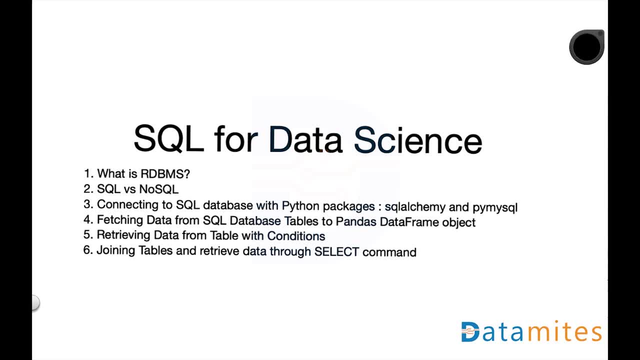 RDBMS, which is relational database management system, And SQL versus NoSQL is the differences And why SQL or NoSQL preferred for a certain applications. And we dig into connecting to a SQL database with Python packages, SQLAlchemy and PyMySQL, and then we look into fetching data from SQL database tables to pandas data. 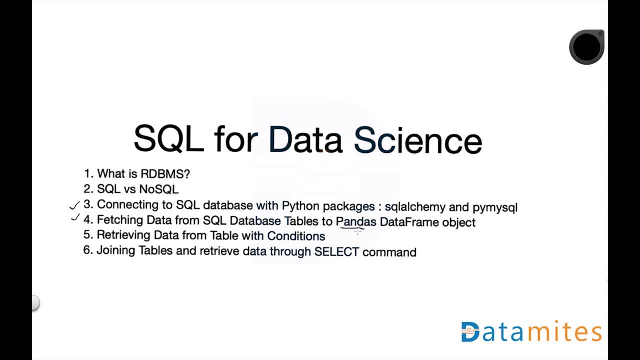 frame object and, as you know, pandas is a base package for all data manipulation in data science, base package in Python. so I'm assuming basic for basic knowledge or a knowledge in pandas and if you don't have the knowledge in pandas package then I suggest to click the video given in the URL in the 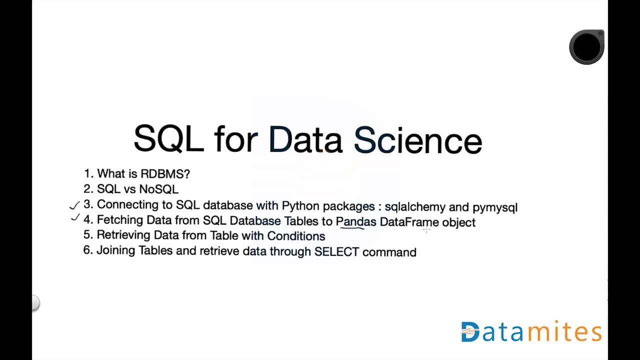 description and, and you know, complete that pandas tutorial and and revisit this sequel tutorial. and then we go into retrieving data from table with conditions where condition and also logical conditions, logical operators and an hour, and then we go into the joining tables and retrieve data through select command. what we don't discuss in this, in this session, in this tutorial, is: 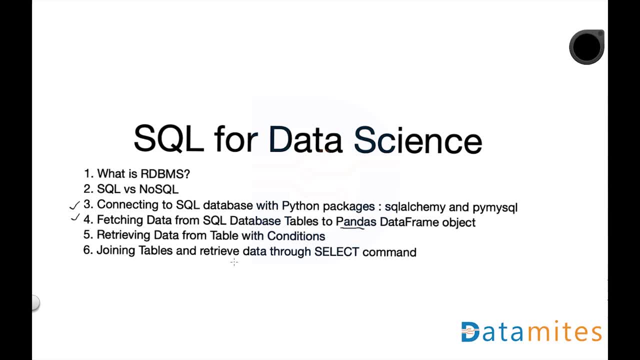 a. we're not going to update the data. they update the tables, create databases, create tables, structure them and all the stuff, because that's more into the for the software development. so if you're developing an application, you need to do to structure the data: write, update, delete. for data science we are mostly 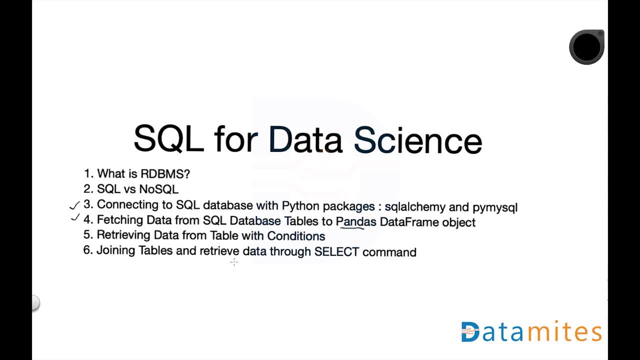 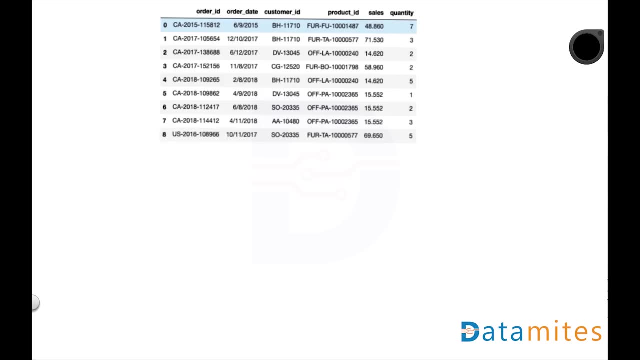 concerned about retrieving the data from the databases, so select command is the one which is. it's relevant for us all. right, let's get started. so this is a table and this table is is is an order stable. so it's imagine an online store, online store, and this table is orders. it has order ID or the date. 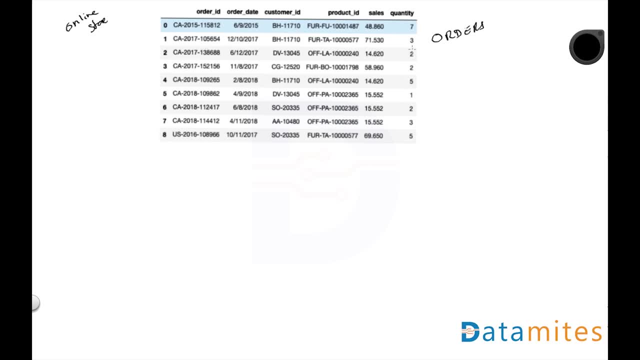 customer ID, product ID, sales and quantity. I have made very few columns or the fields because I want this exam to be simple, but but but in practical you have 1520, even more fields in order table right. so what you observe here in the customer details we only have customer ID, for example, your BH, age and 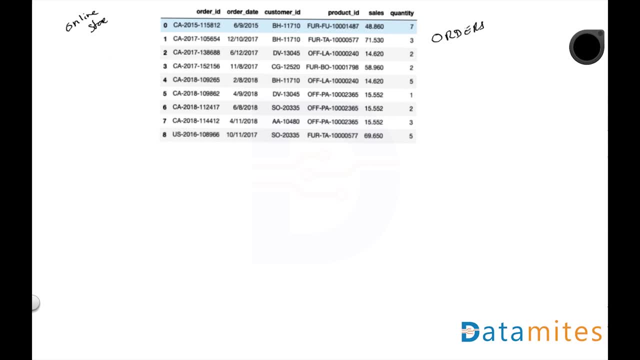 1171001.. and it doesn't have any other information and this information is stored in- it's a separate table called a customers table, okay, and this contains, for example, this: BH: BH 1 1, 7, 0 has. here it is, it's a customer name, is: 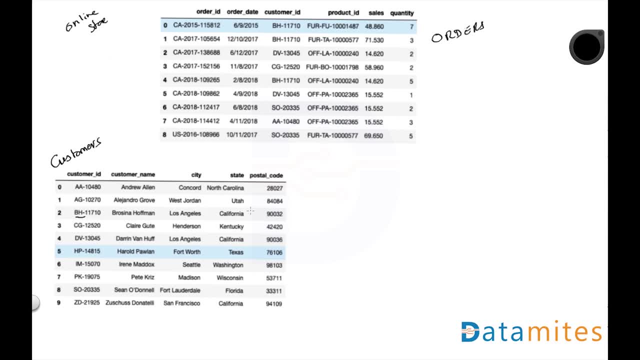 Rosina of man. it's Los Angeles and California and the pin code is 9 0 3, 2. why do we do this? well, one of the main reasons we do this as a part of this RDBMS concept is saving a lot of space. let's think about it if you put these: 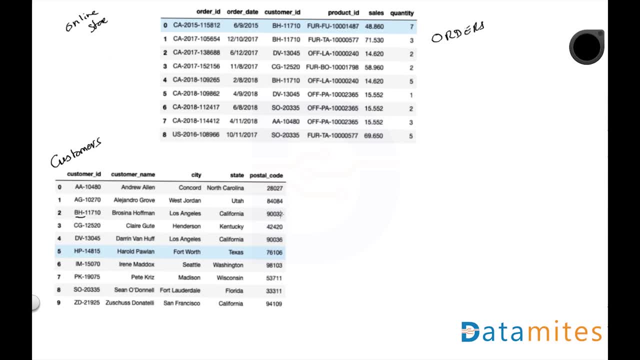 details: the customer name, city, state and pin code. and just to remind you, this is only few fields have selected. that might be 10, 20 fields related to the customer and this basically comes over here, right? and if the customer buys an another product from the online store, something. 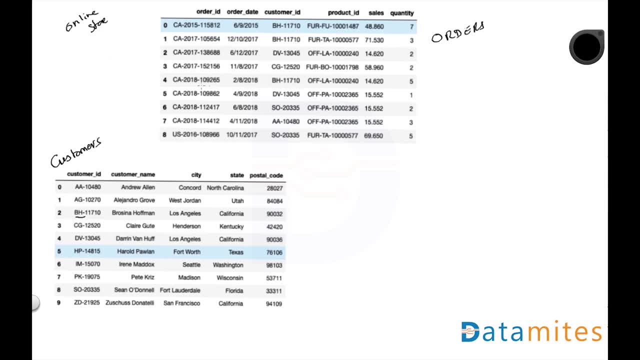 like this. even the second record is from the same customer. even even the fourth record, I would say it's fifth record starting from zero. so fifth record, the three times in this nine records this customer has actually repeated three times. right, rather than customer ID, it's start. if you start putting all the details of the customer, it will occupy a 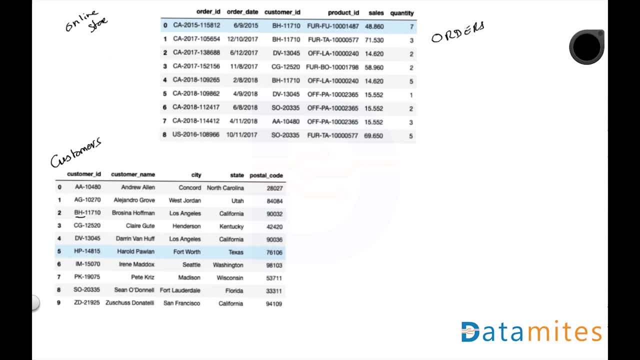 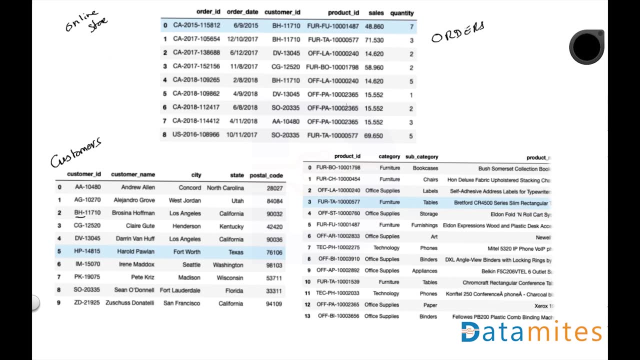 lot of space, right? the same goes with your product ID. so, rather than putting a product ID, if you put the product details itself. every time someone orders a product, for example, you have this: Oh, FF LA 240 1 0 0 0 0, 240 is appearing over. 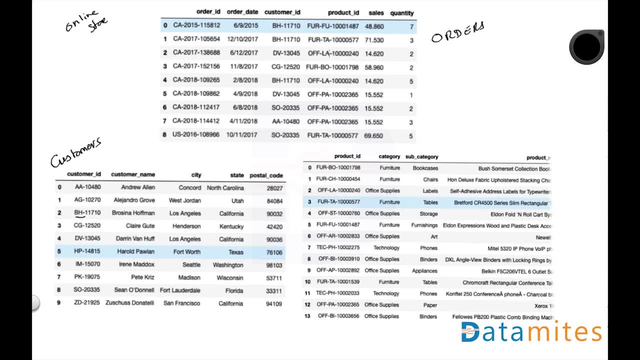 here as well, right? so every time someone orders this, this product, you have to really put the entire details of the product and this is it's. it's really a lot of space and if the transaction runs into millions of records, there will be a massive, exponentially high of storage is required to store it. this is 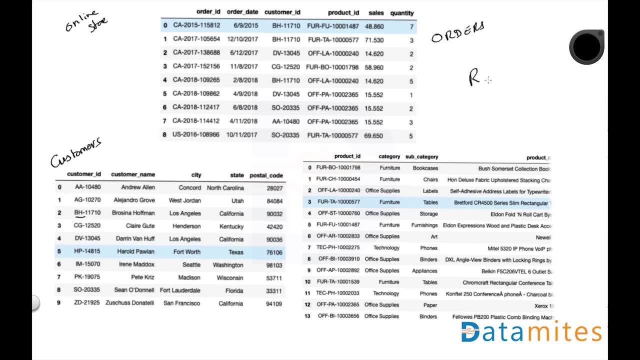 the main advantage of this rdbms relational database management system, and even today, when i say today, i'm talking- uh, it's year 2019. rdbms is the highly used database system in the world. right, well, it's called a sql, because sql is is is a structured language used to retrieve data. 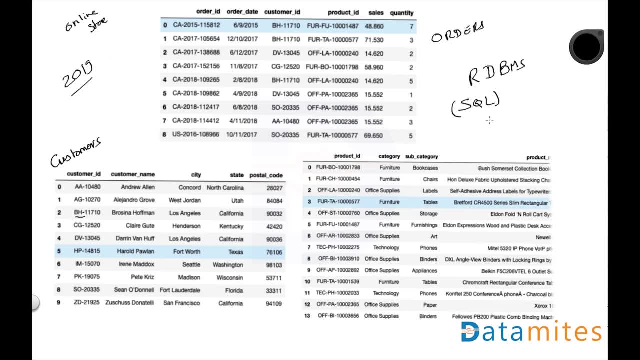 manipulate the data. in fact, in general, managing the data in the rdbms system- no sql, which is the the the alternative of it- has gained a huge popularity in recent days, for the simple reason that you don't have to have many tables, and connecting all the tables. 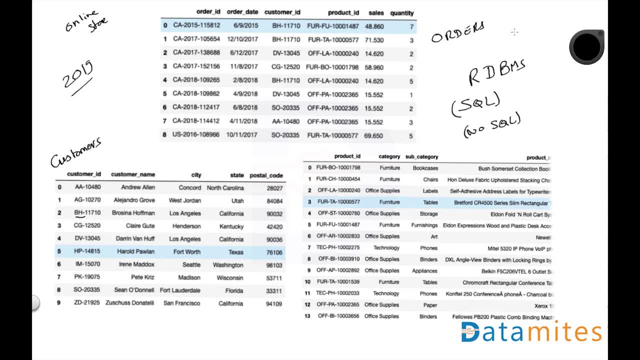 we store the entire transaction in just one record, well, well, that has a disadvantage of having a huge storage space. that's the whole reason we have rdbms, right, but well, given, thanks to technology breakthroughs, given that we we have no real constraints of the memory, so we 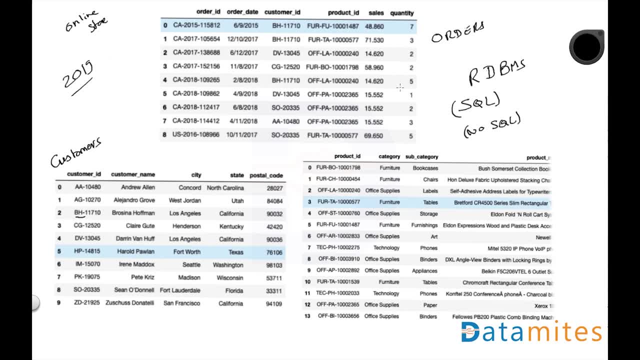 have huge memories. megabytes, terabytes- can be stored. this made it possible for no sql to become popular. no, sql actually consumes a lot of memory space, but given that no sql is better in terms of the retrieving fast and it's highly scalable, right, no sql is gaining popularity, it's it's faster. 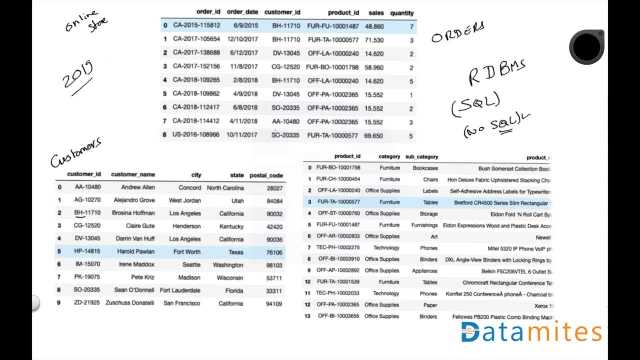 because look at the sql, so it has to really connect. i mean, basically when you run a query, your orders has to connect to the customer with the customer id and connect to the product table with the product id, retrieve the data, then get the full information. in no sql, all the 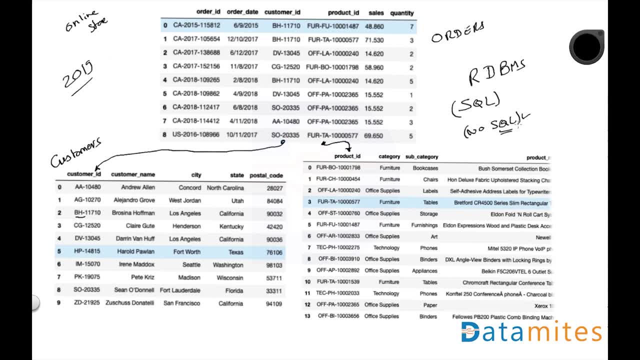 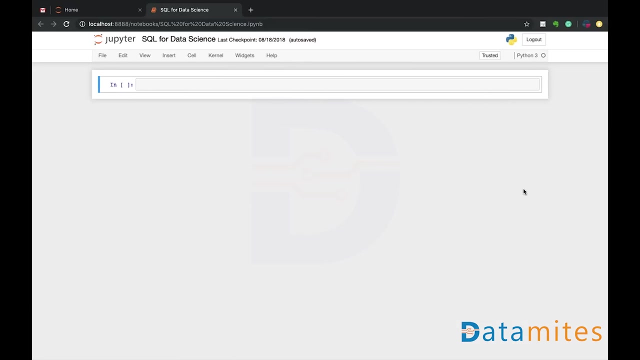 information is stored in just one flat record. all right, that's the major difference. i shall record in another video with a very detailed differences between sql and mysql. let's move ahead and look into how do you actually connect to the sql database using python. all right, so i have a blank jupyter notebook again. if you're not very aware of jupiter. 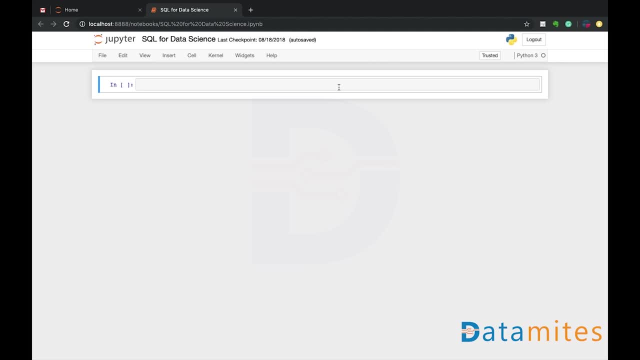 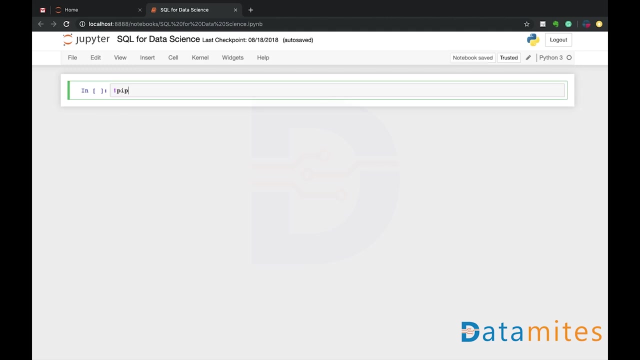 haven't used it. i have another video. also mentioned that in the description. please watch that video and come back to this. jupiter is a notebook, it's a. it's a platform for data science development. okay, and the two packages i have mentioned is pip install, sql, alchemy. 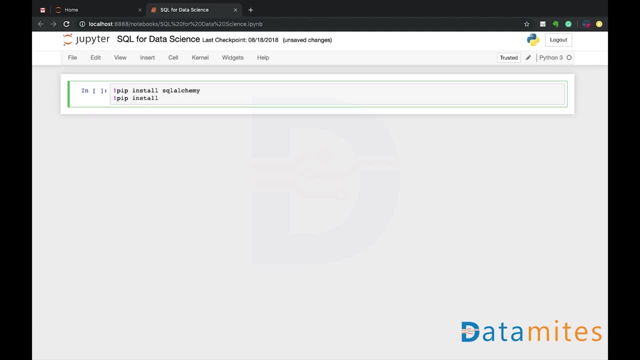 and pip install py mysql. just run this too, and the symbol over here exclamation is, is directing the jupiter to run it in the the shell, the anaconda shell. so just running this. for me it says both are already satisfied because they have been already installed. it's of course. 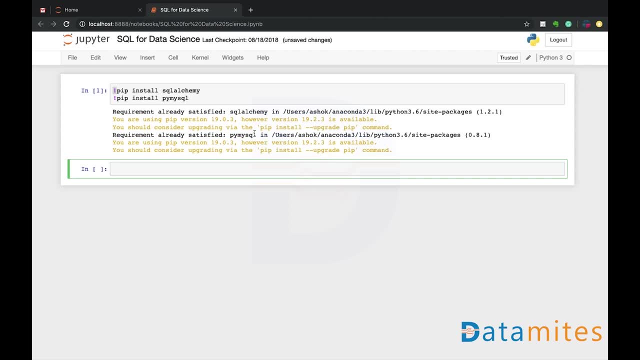 giving me some suggestions about upgrading the pic, but when you install, if you're doing it the first time. so basically it downloads and installs. it's a small packages, it won't take much time, right, and then simply import the packages which have installed. let's see for, from sqlr, our chemistry, sqlrchemy, we import, create engine. that's, that's object. 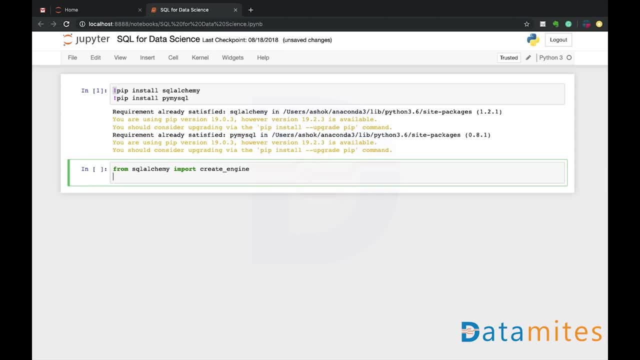 that's the module we would like to use and of course, we go ahead and import pandas and and that's it and um. the next step is to actually get the details of the database. this should be provided by the, by the client or whoever says that you know something is wrong, and especially for 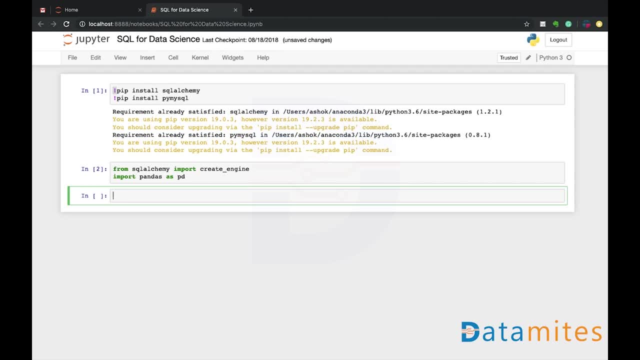 sqlark, my sqlark. its not that good. so that's the second step we take into account now. so whoever is sharing data with you? so I have a test server being set up in data mites test server, and these are the information so you'll be getting. 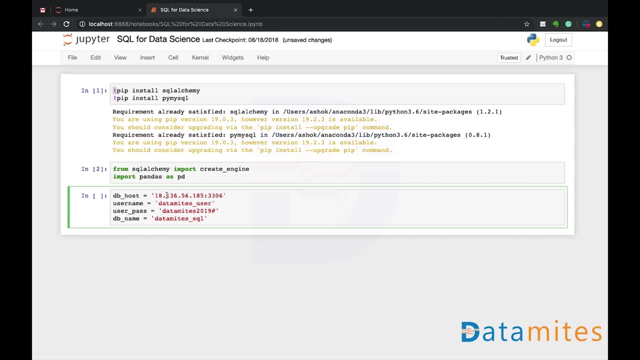 something like the to the endpoint, in this case this IP number, along with the port number, username, password of the user who has access and the database name. okay, I'm just gonna run this and store all these details in the corresponding variables, right? and then I'm going to simply call as connection. 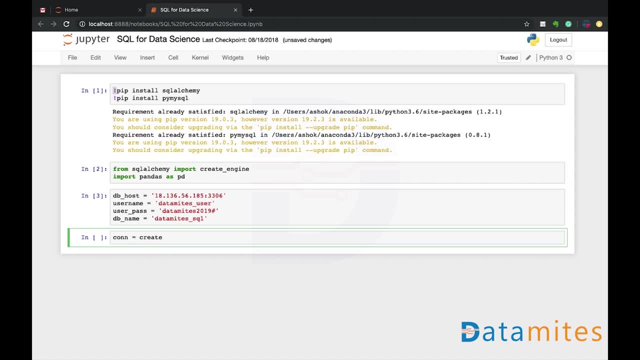 CEO. and then, and I can create a connection by using this object from sequel alchemy, and this is the format, it's mysql plus py sql, and you put a colon, slash, slash, and you can actually give the details. for example, the next one would be a user name. 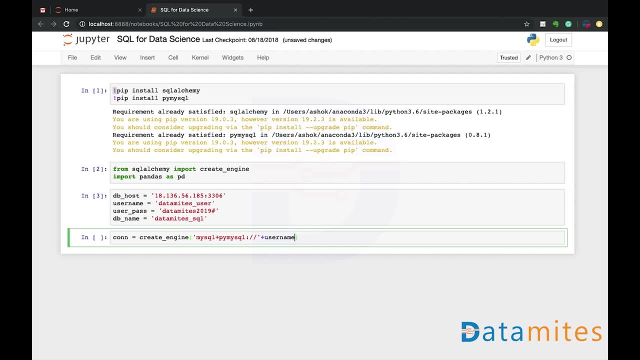 and after username you need to put a colon, so you can do that by this and say plus. by using plus we are concatenating the string. I'll say pass and then just be careful not missing a common quotation, and next is actually host, host, and then you need to use a forward slash and then dvname. so this is. 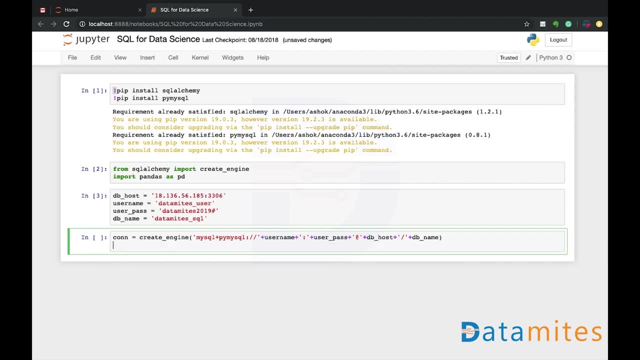 your connection string and- and this is actually creates a connection string, let me say table names and this should actually give you table names. just running this should give you table names. let's try that. okay, and I didn't know arrows. okay, always land up errors in my names, I believe. let's none. Lab delegated. 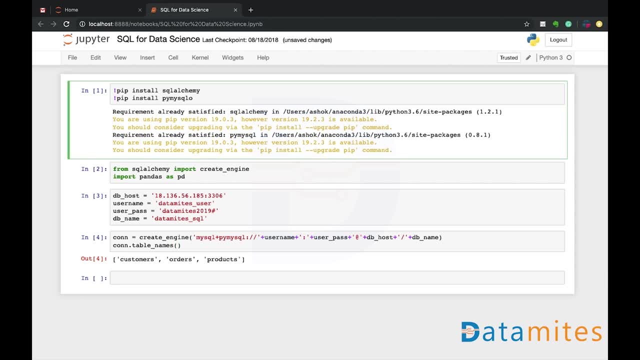 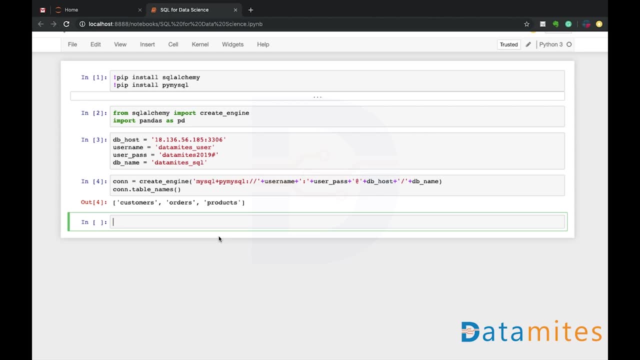 me again. now see at the day: what do we do we remember? how many hours does it paper run 옛날? first it says cog lady say first D. now I'm going to set this up, since the word home, party, Пол, land up errors and then we fix it. but lucky, we got no errors. so we have three tables. 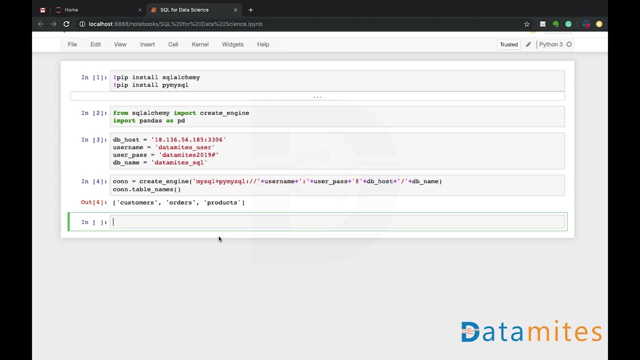 orders, customers and products- very similar to what you have seen in the whiteboard explanation. let's first connect to the orders table and retrieve the data, and that we do it by using creating a query sting again, and this is what we call it as sql query right and we are focused on 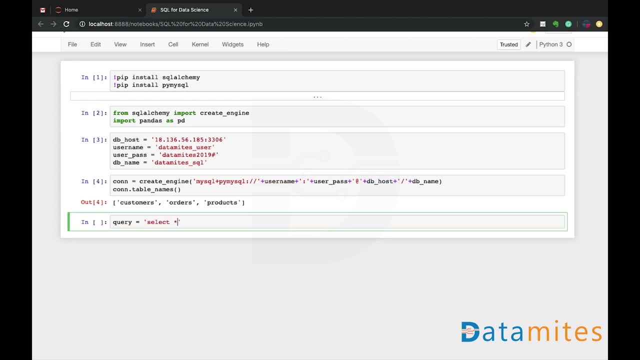 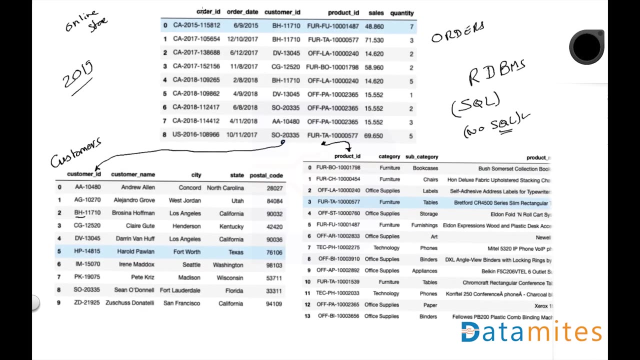 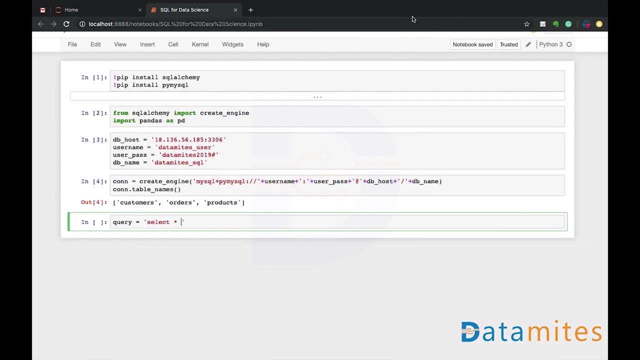 select. so i'm going to use select. so when i say select star, it selects all the fields. for example, this is the table we are talking about. so i'm saying, give me all the fields: order id, order date, customer id, product id, sales and quantity. i say star and say from and i simply mention the. 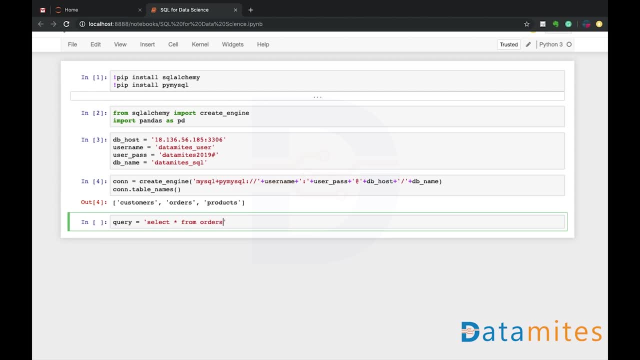 table name orders. okay, and this is a query. i mean, this is a simple string and then i run this query like pd dot read sql, because i'm using pandas to run a sql query and i simply pass on the query and then i pass on the connection so it connects to the database using connections connection. 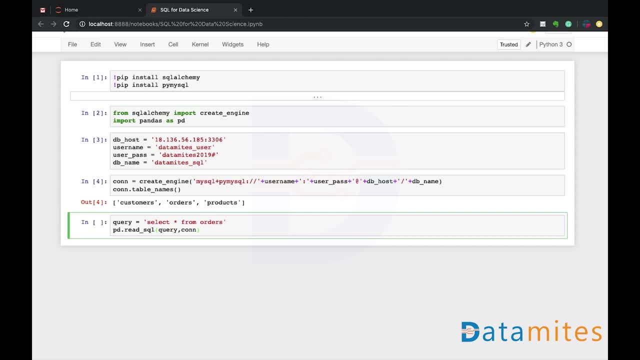 the connection object and the query string is given over here. it simply runs and returns the data. let me capture this data into a orders- orders variable and this will be a data frame. okay, and let me just print down the orders shape, just to know what is the shape, and then i can simply print down the orders itself. 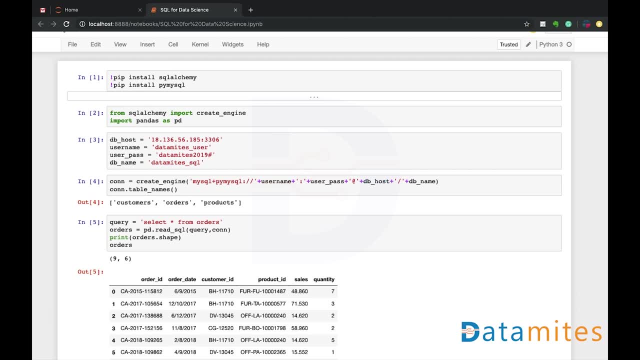 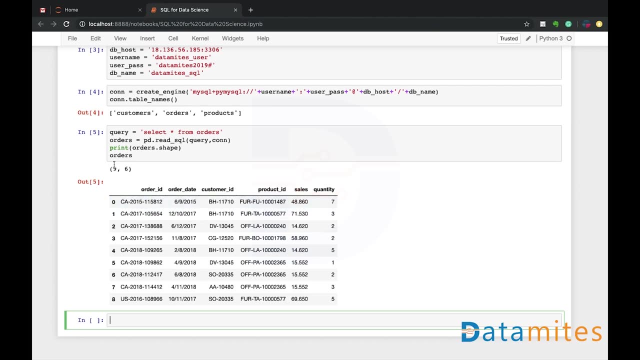 run it it might take. oh, it didn't take much time. very small database so it didn't take time. so we see that we have retrieved the entire database, in fact the the entire table. in the table you have nine rows, zero to eight, nine rows, six fields or columns, because it's right now, in, in, in, in, in. 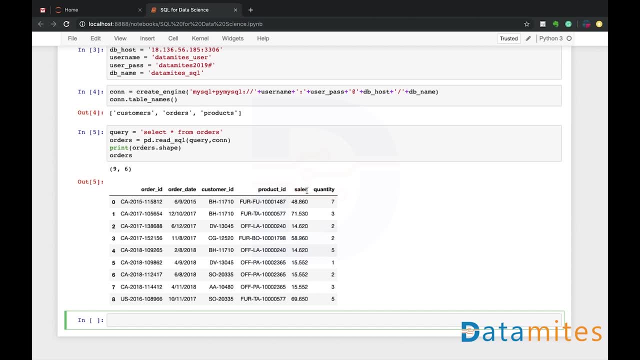 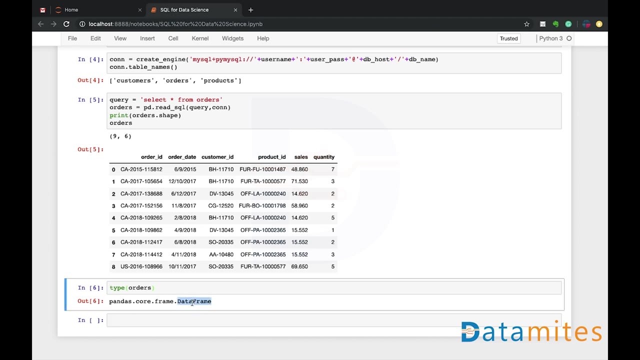 data frame: order id: order date: customer id, product id, sales. just to see the type of this order, you'll see that it's a data frame because it's been retrieved by pandas. pourquoi function? you see, it is actually a panda score frame. data frame object. okay, here we go. so it is actually. 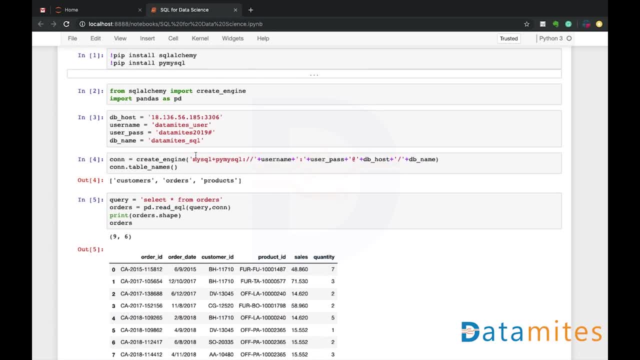 that simple to connect and you really don't have to remember this and just have to, you know. copy paste this string and make sure that we show all the rows containing the f to get our data frame. okay, 우리는 ríçeci di brace dat. pananya data frame. 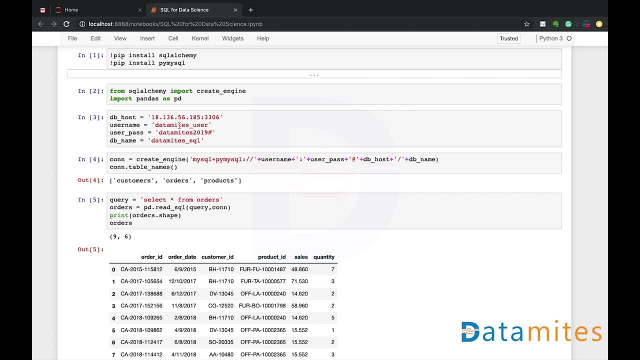 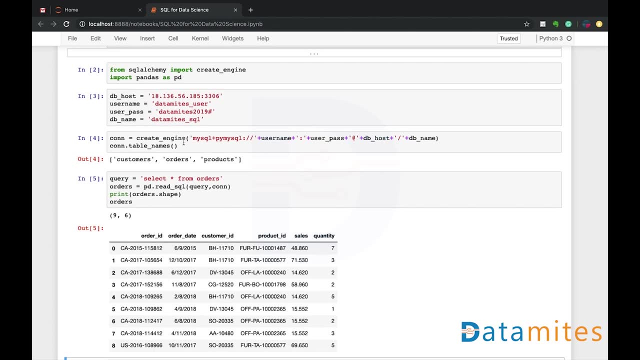 string and make sure that you put the right hostname, username and password and also mention the DB name. and you don't have to really know the table names, because that can be simply retrieved by using a table underscore names function from the connection. it gives you all the tables in the database and then you can. 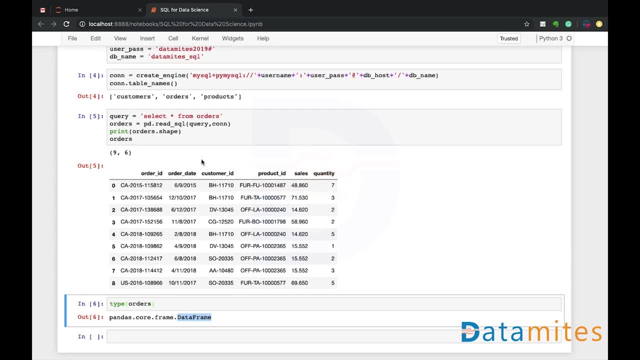 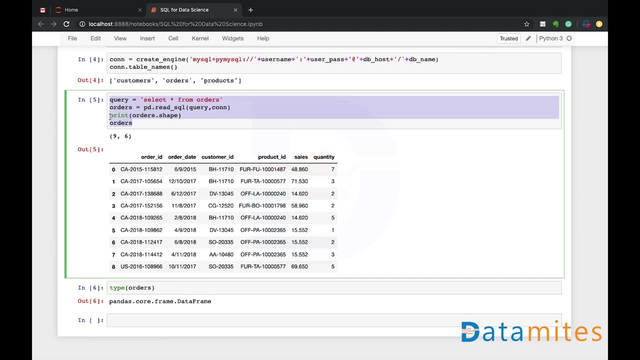 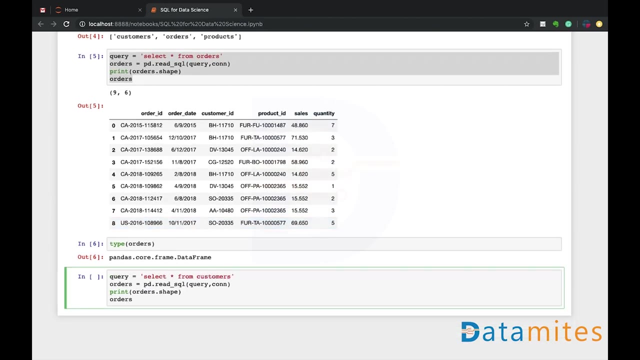 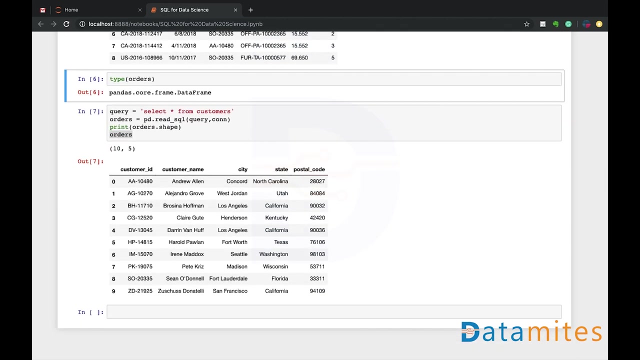 use a select command, the query, to connect to the table and retrieve all the records and store it in a data frame. okay, we can actually repeat this for for other. for example, let's say do it for customers and see: okay, sorry, okay, so let me keep that: orders, orders and for customers, I call it as customers itself.